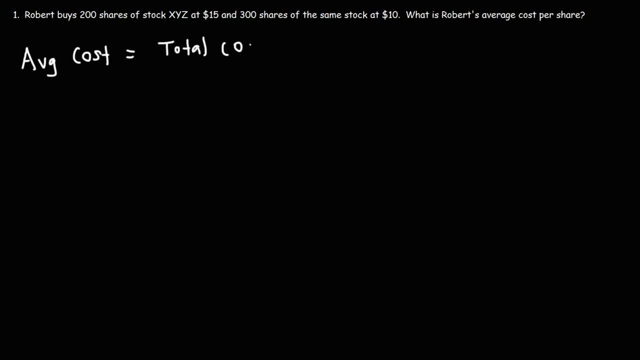 the total cost divided by the total number of shares That he owns. So first let's calculate the total cost. Robert purchased 200 shares of stock XYZ at $15.. So if we multiply 200 by 15, that investment is worth $3,000 at that time. 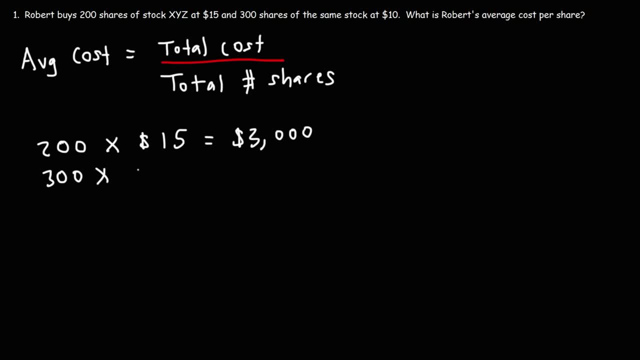 Now he also buys 300 shares at a price of $10. So which means that he also invested $3,000 during his second purchase. So his total cost in buying these shares is $6,000.. Now the total number of shares that he owns is 200 plus 300, which is 500 shares. 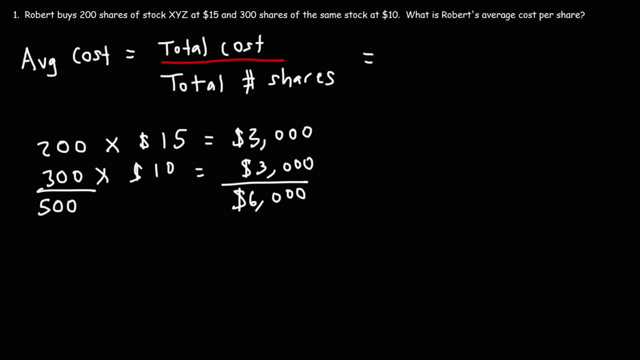 So that's his average cost- is going to be- Well, let me write that here- His average cost per share From these two transactions. it's going to be the total cost of 6,000.. Divided by the total number of shares that he owns, which is 500. 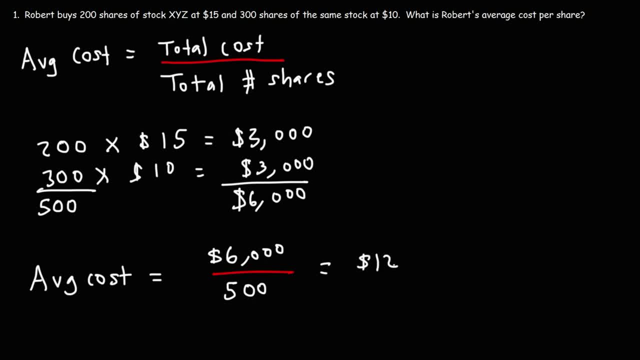 So his average cost per share is $12.. So note what happened. Initially he bought the stock at $15, but when the stock fell, he bought more shares at $10. And so by buying the stock when the price went down, he was able to reduce his cost basis or his average cost per share in that stock. 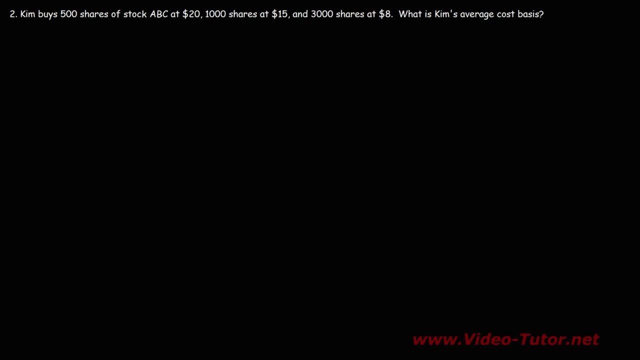 For the sake of practice, let's work on another example. problem Number two: Kim buys 500 shares of stock ABC at $20,, 1,000 shares at $15, and 3,000 shares at $8.. What is Kim's average cost basis? 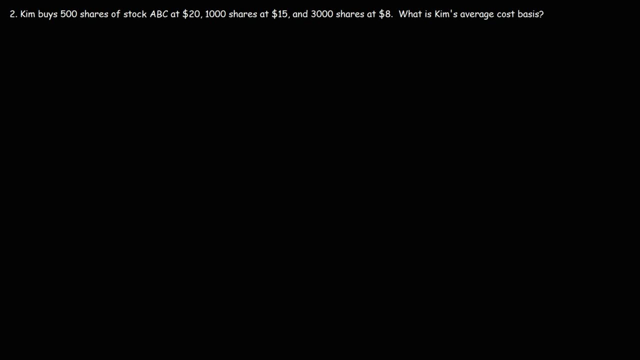 Or rather, what is her average cost per share. So we're going to follow the same exact process. We're going to calculate the total value of each purchase that she made. So in the first purchase she bought 500 shares at $20.. 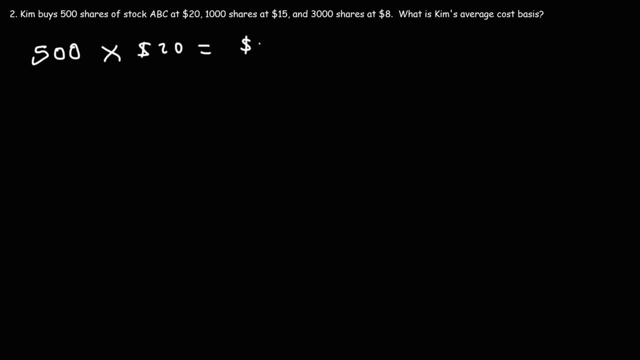 So 500 times 20 means that her first investment was worth 10,000.. So she bought 1,000 shares at $15.. Now for the second purchase: she bought 1,000 shares at $15.. So the value of her second investment is 15,000.